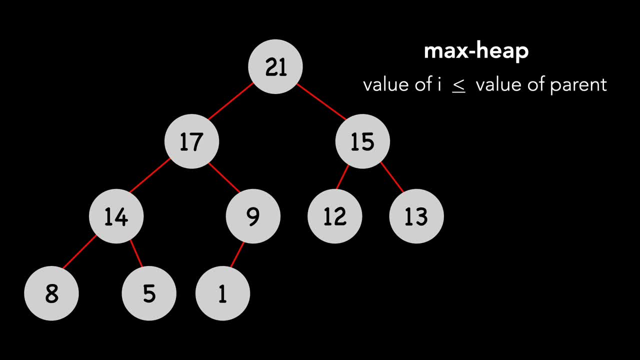 value of the node i is greater than or equal to the value of its parent. Max heaps are used for heap sort. Similarly, for the min heap, the value of the node i is greater than or equal to the value of its parent. Min heaps are great for priority queues, Because we said, heaps are nearly. 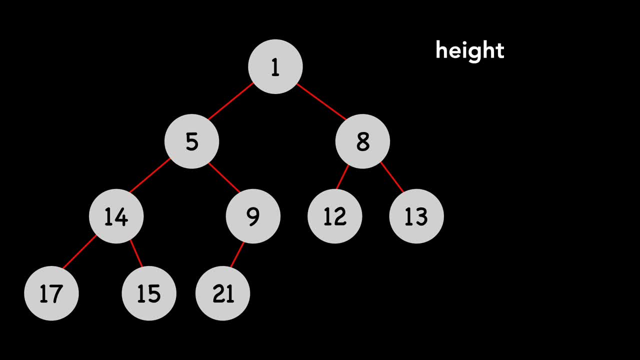 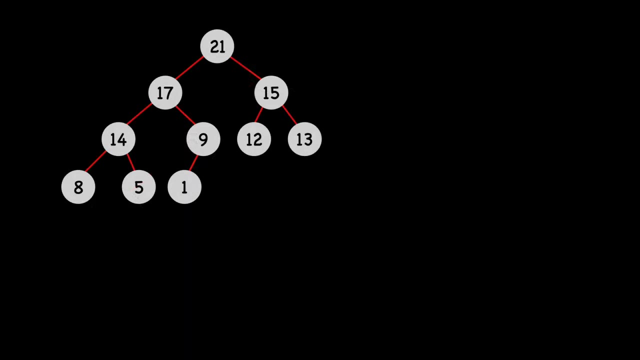 complete binary trees. we know that the height of a heap is O, which you'll see in various operations that we'll learn later. I'd also like to show heaps represented as an array. Here's our max heap and here it is as an array. The root of the tree is at index one of the array. 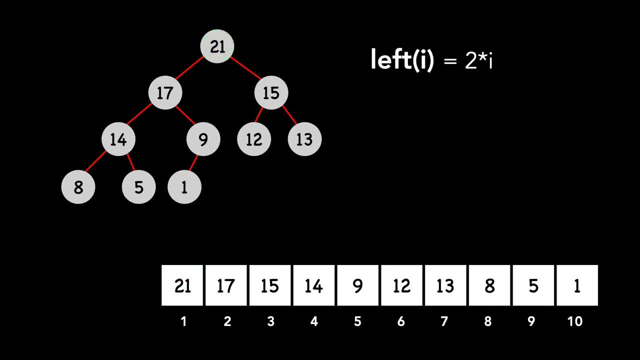 To get a node's left child, you simply take the index times by two. And to get the node's right child, you take the index times by two and add one. Finally, to retrieve a node's parent, it's the floor of the node's index divided by two. We choose to put the root at index one instead of zero, as it. 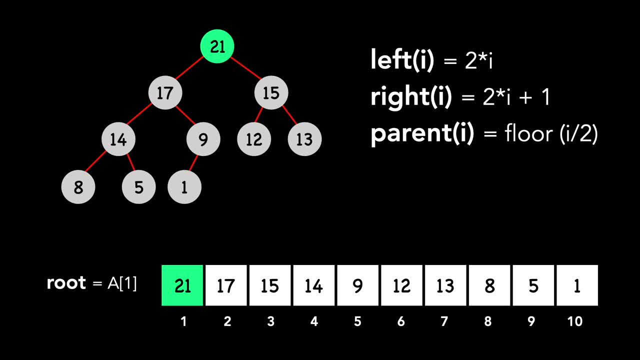 keeps this array in the same order as the root of the node's parent. The root of the root of the node is arithmetic cleaner and most computers can do these operations with fewer instructions. Let's take a look at fifteen, which is at index three, The left child of fifteen. 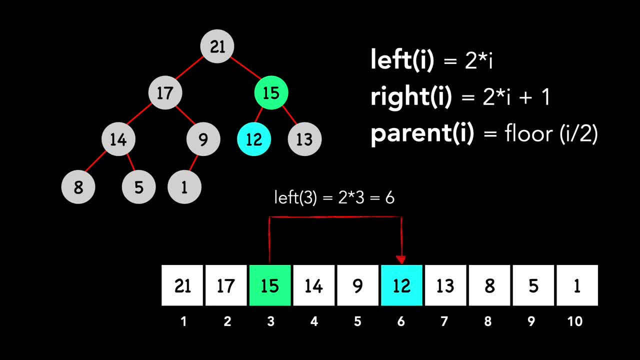 is equal to two times three, which is the sixth index, and a node value of twelve. The right child of fifteen is two times three plus one, which is the sixth index, and a node value of twelve. The right child of fifteen is two times three plus one, which is the index of seven or the node thirteen. 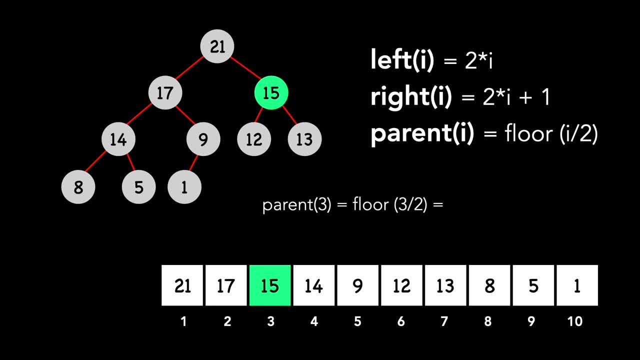 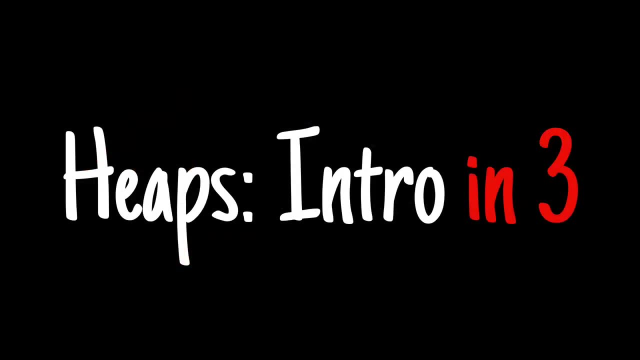 Lastly, the parent of fifteen is the floor of three divided by two, which is the first index and the root of our tree twenty-one. You know I prefer brevity, so we'll end the video here and in the next one. 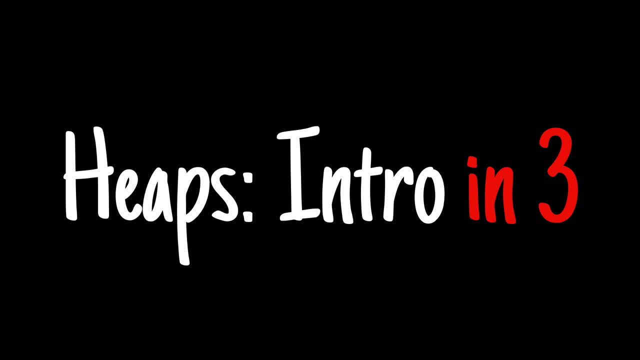 I'll show you how to create a heap from an unordered array. Thanks for watching. I'll see you in the next one.